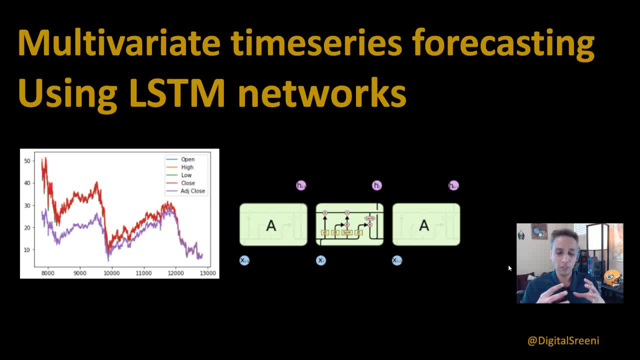 have only one data and you're trying to forecast based on that one data. okay, That can be stock price or in fact, in the past we looked at airline passengers: how the passengers- you know the number of passengers- actually change or increase or decrease with respect to time and how we can. 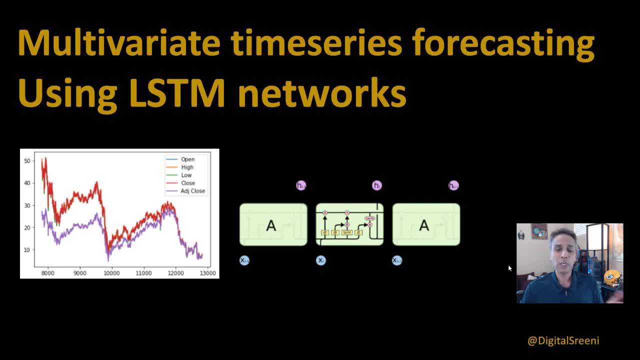 forecast that. So here is an example where we'll do exactly that. So not many tricks actually. If you understand that, then you should be able to understand this in an easy way, except instead of one variable we'll have multiple variables. That's pretty much it, okay. 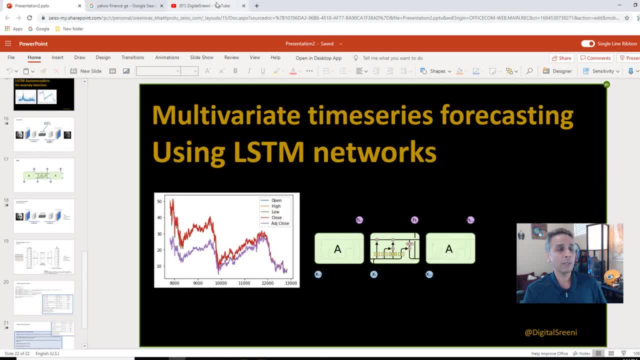 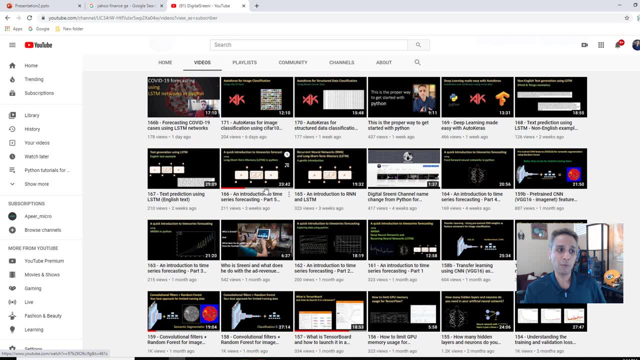 Now let's jump into it and, as usual, I'm going to use Python and Keras. but one thing I'd like to highlight is again watch videos 165 and 166, because they provide some introduction in case you already don't know what LSTM is and how to use it for time series And for today's video. obviously I need some sort 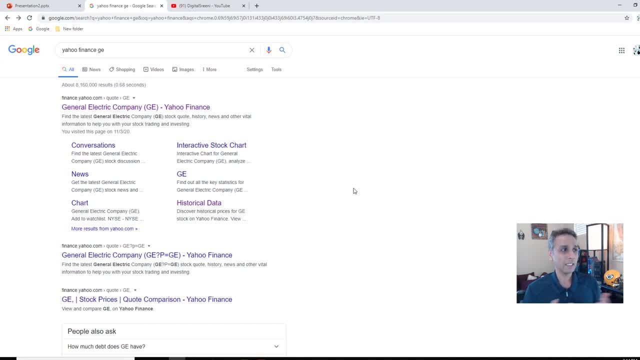 of a multivariate data set, and the best thing I thought would be stock market. Of course, if you have other data sets, please go ahead and use it. This is the best one I can think of, especially because we used exactly the same data in the previous video. Right now, the 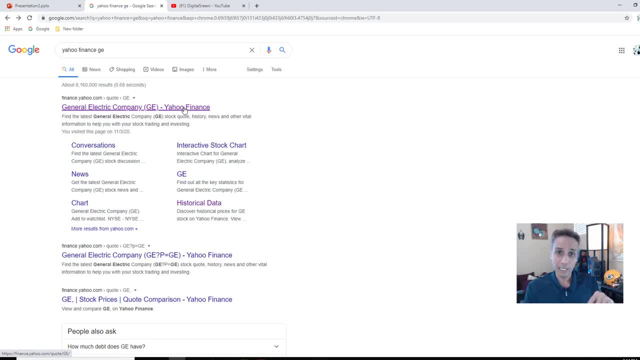 video before this one where we did auto encoders using LSTM auto encoders and we looked at reconstruction error and looked at anomalies in the data. So this is exactly the same data set, except instead of only looking at the closing price or opening price, let's go to historical. 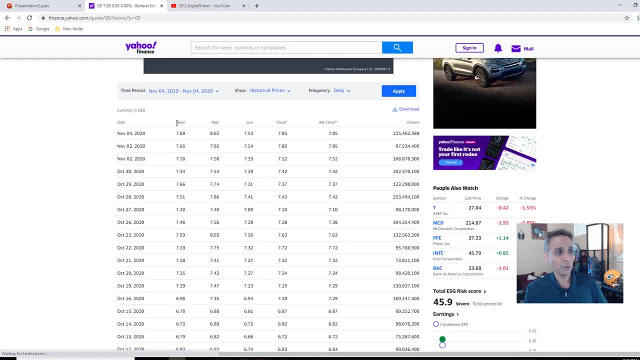 data. So it's going to show us a whole bunch of data. So for each date we'll have the opening price for the stock market, For the stock here, high, low and close and adj close. I have to look down exactly what it means. 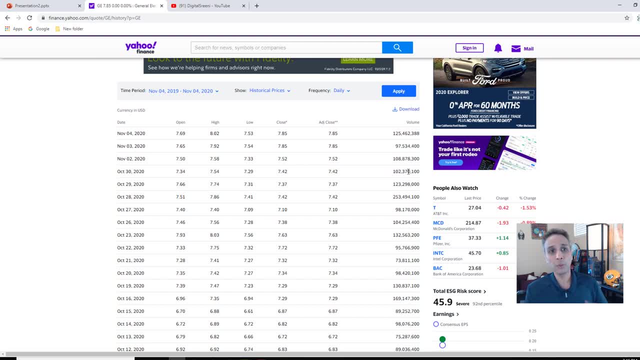 and also the volume. I don't think we'll be using volume, even though you can use it, because we'll be normalizing the data sets. So what the plan for today is use these one, two, three, four, five columns- okay- as variables, including the first one. okay, all of these as variables. 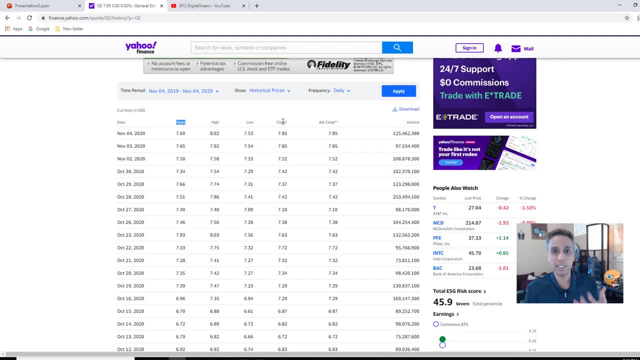 to predict the opening price. We can also predict the closing price, it doesn't matter. Let's predict opening price using all of these as variables. So we have five variables and one thing: one of those is some what we are trying to predict and the assumption is okay. so 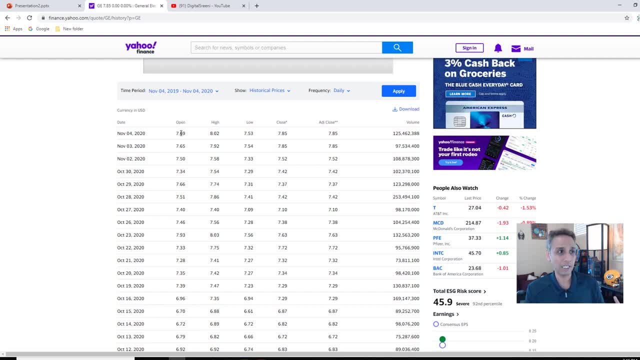 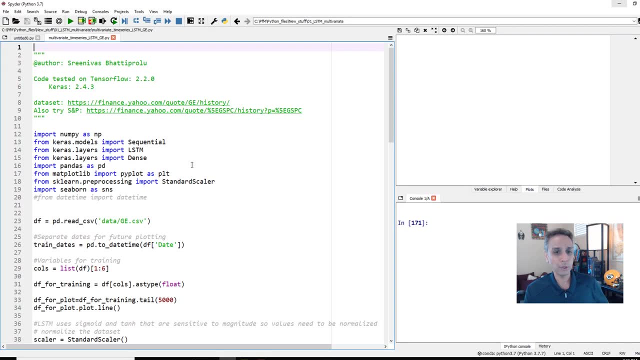 these are the right variables that are affecting the price, you know, for the open price. Okay, so with that knowledge, let's just go ahead and jump into our spider IDE and I have tested this on TensorFlow 2.2 and Keras 2.4.3, but there is no reason it doesn't work on the open price. So 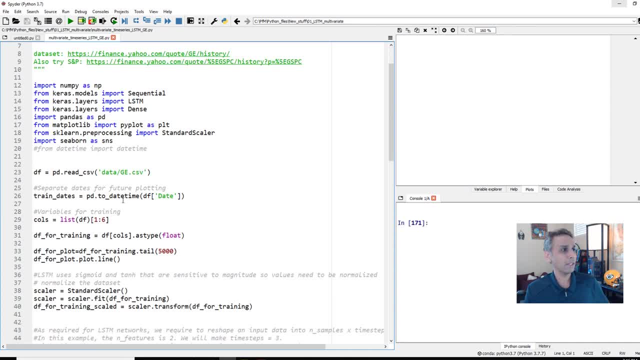 let's test it on other versions. okay, Now let's go down and import our libraries. These are pretty much the standard ones. no tricks here. We are importing LSTM and dense layers, because these are the ones we are going to use, and using Keras models sequential method, we are going to put 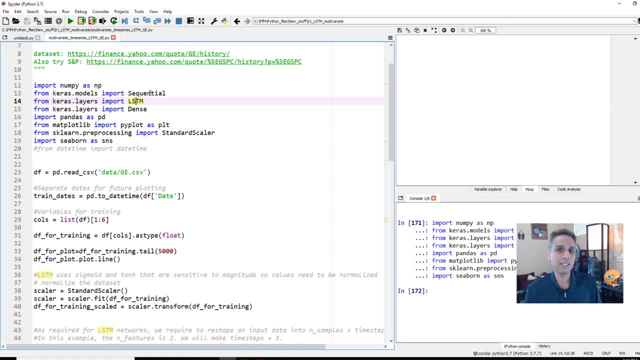 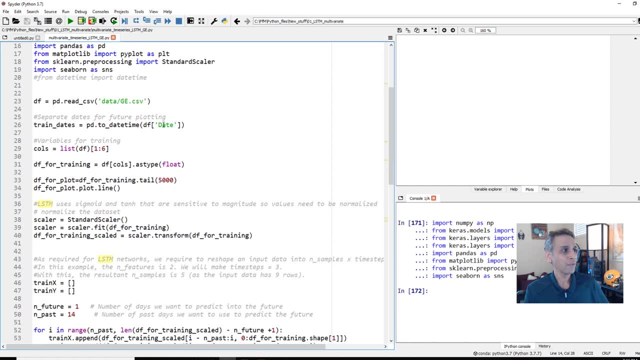 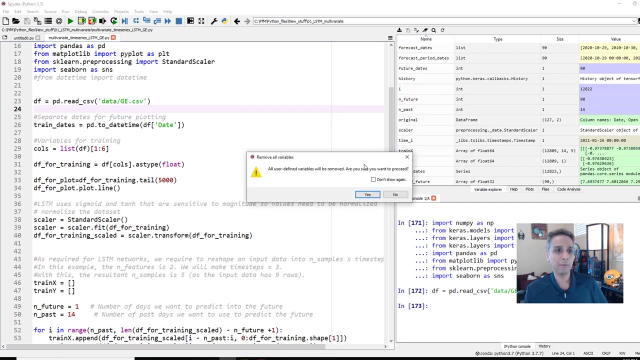 together our LSTM. That's the easy part. The tough part is getting the data ready in the right format. Once you have it, then this is pretty much straightforward. Okay, so let's use pandas to CSV file and let me switch to Variable Explorer. Remove all variables here from my previous runs. 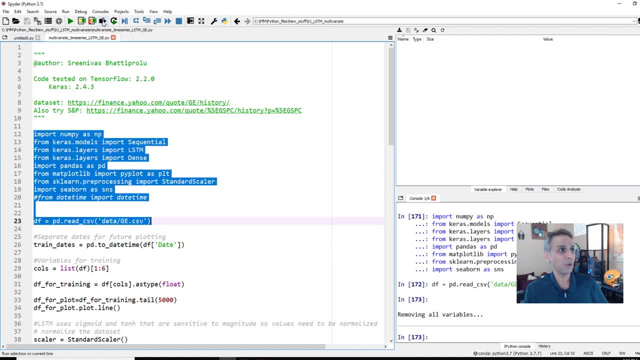 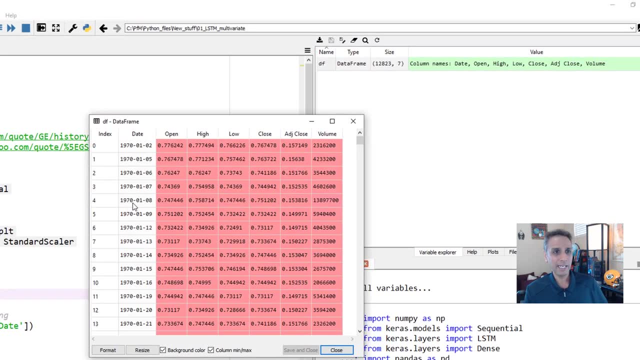 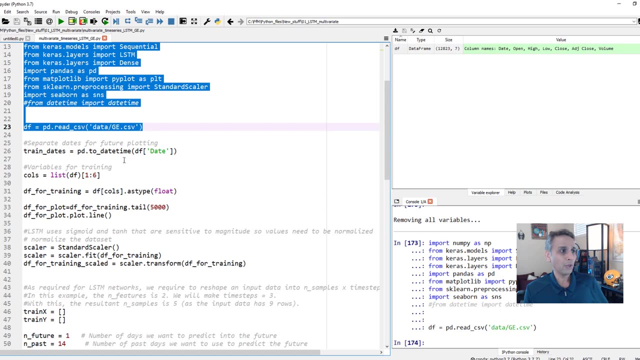 I was testing something else, and let's run these lines one more time. Okay, so now it's very clean. So our data frame should have seven columns: One for date, the five variables we talked about and the volume- Okay, number of transactions that day, Okay, so what shall we do now? So if you look at 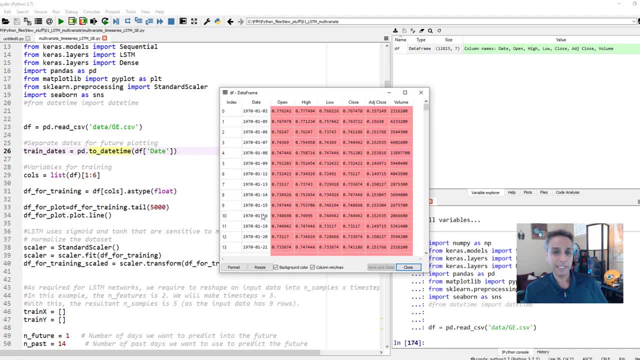 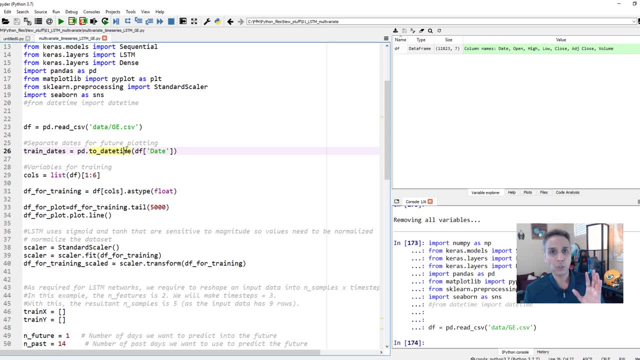 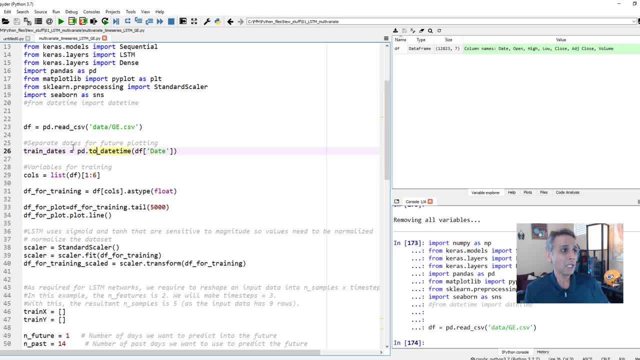 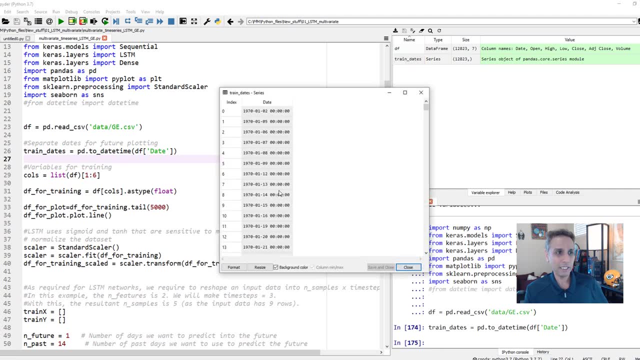 variables. date is not one of the variables, right? So what I'm trying to do here is extract the training dates into a separate series So you can see the training date right here. So later on when we plot we can use that as our x-axis. That's pretty much it. Okay, so that's the reason I. 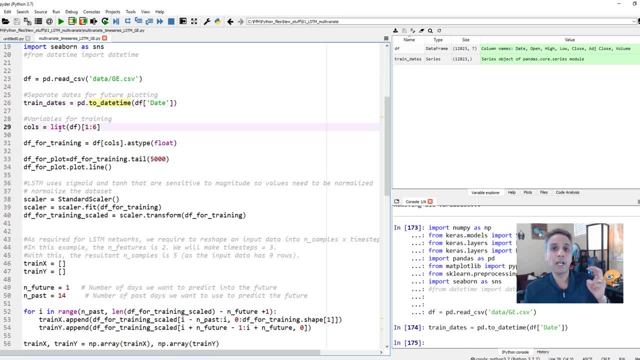 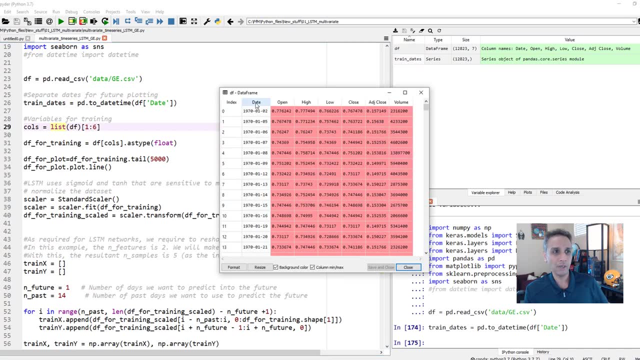 wanted to do that, And now let's extract the columns that we would like to use as variables. So these are the columns number one through six in our data frame, right? So column number zero is our date and one through six is one, two, three, four, five, six, actually including the volume. Okay so, 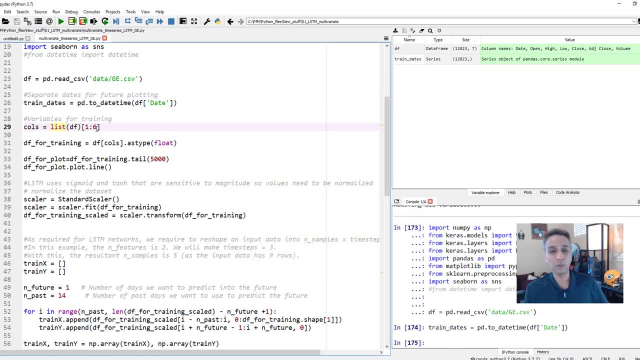 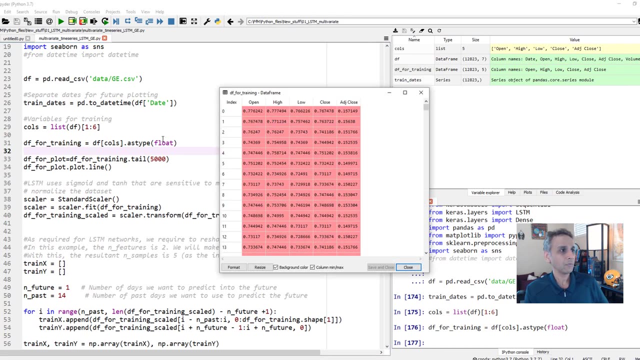 let's go ahead and include these. Of course, you can go one through five if you don't want to include the volume, but let's just include it for now. So let's go ahead and do that. And now, for example, I'm just creating another data frame and again you can see: oh, this is excluding six, So I'm 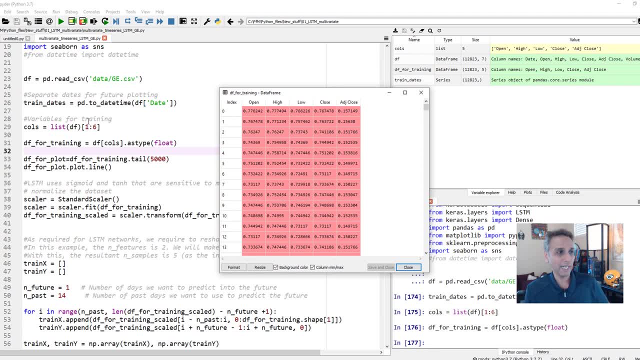 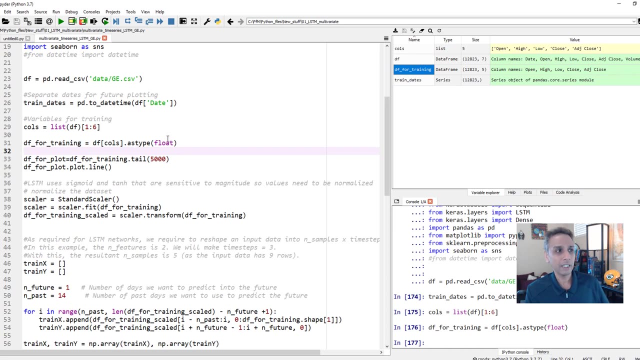 not including the volume. I always forget that, Anyway, so our new data frame is basically the old data frame with these columns without the date and the volume, right? Okay? so this is our new data frame and I converted all the values to float. so when we actually do normalization, you don't lose. 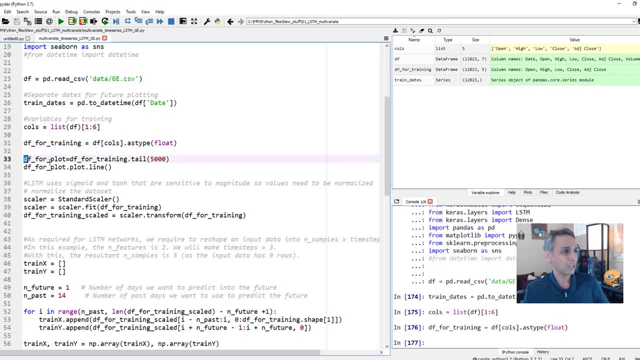 any information there, You can plot it. I was doing some experimentation. They aren't. all I'm trying to do is: okay, let's look at last 5,000 data points and see how they look like, but it looks very boring, So let's go ahead. 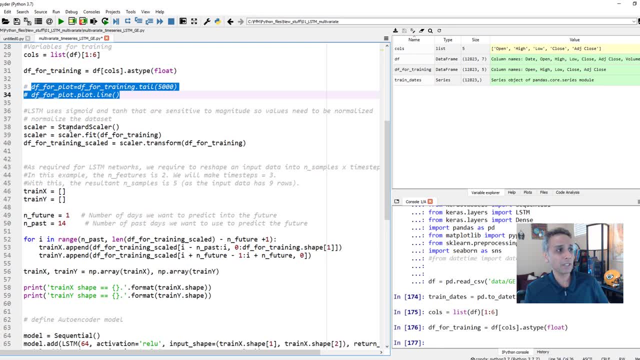 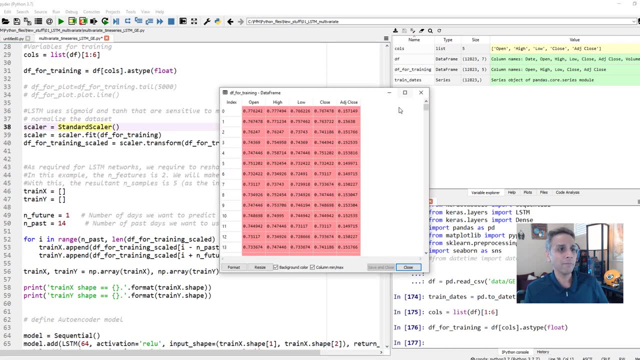 and comment this part out. The next step comes as scalar. Okay, so again you know why we are doing this. because let's go back to our data frame. You can see the values look like they're all very similar, but if you actually keep going down, well, in this case, 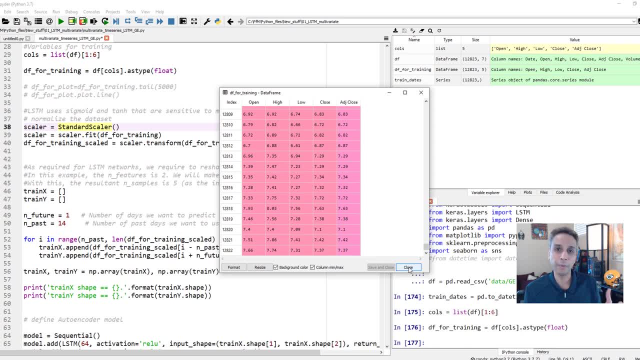 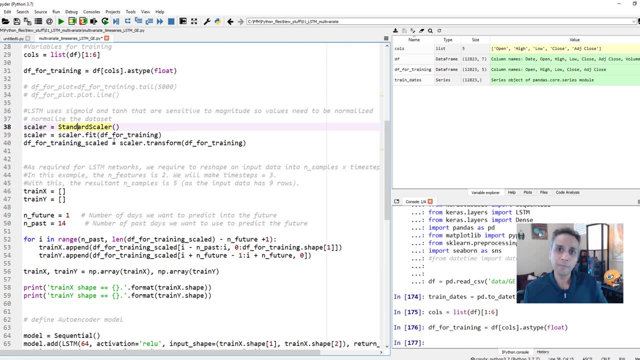 they are similar because they're all the closing and opening, so they're very similar. but scaling them is always a good idea. If you especially include the volume column- yeah, where you have those in hundreds of thousands, because that many transactions happen in a day, then scaling. 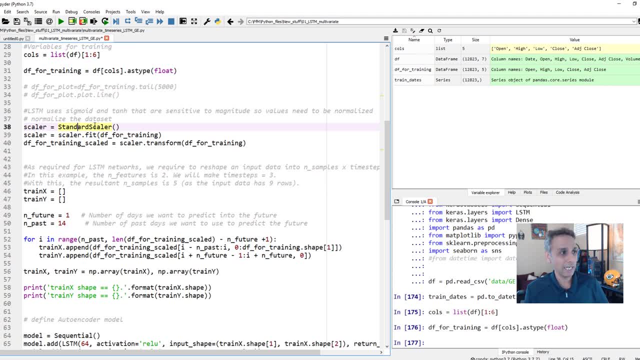 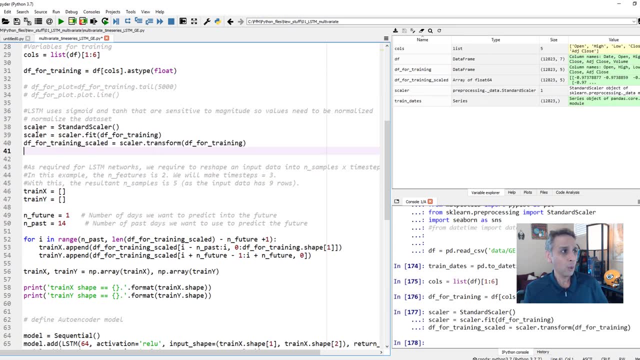 the values is even more important. So all I'm trying to do is use the standard scalar and scale all of these. and you have to keep in mind one thing: When I do standard scalar, I instantiate this and then I'm fitting this scalar using the data which is available as part of df for training. 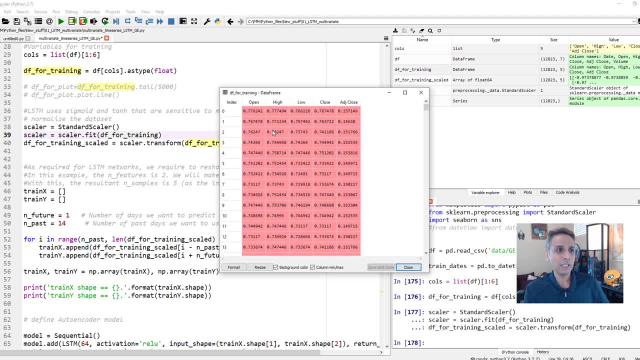 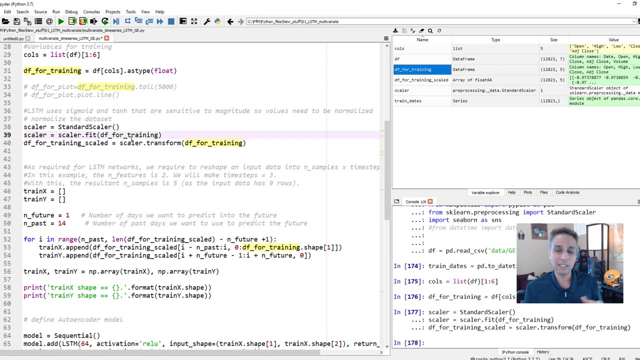 So if I open this data frame for training, okay, it's going to use all one, two, three, four, five columns to do this. I could have picked only one column. The reason I'm stressing a bit on this is later on, when you want to do inverse scaling, because once we scale this, the values are between: 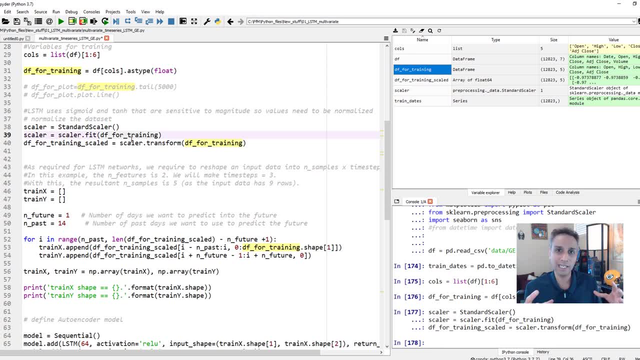 I don't know, minus one to one or minus two to two, depending on how our data is. So this is our data set, but then later on, if you want to get the original data back after the predictions, okay. the inverse transform expects the input to be five columns, because we are using 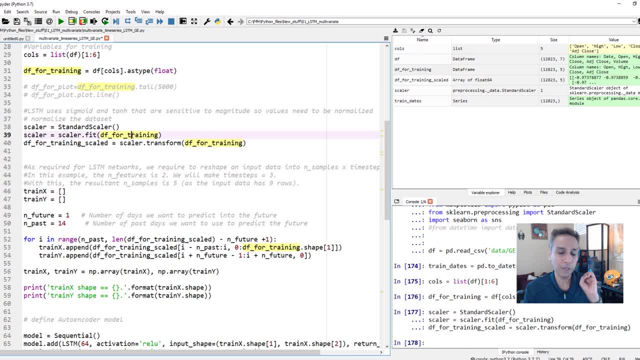 five columns here. Sorry for dwelling too much time, but I'm pretty sure you'll run into some issue if you are not familiar with this, and then it takes a while for you to figure out why it's going on. So if you want to fit it, you can actually, because all of our data is within the same range. 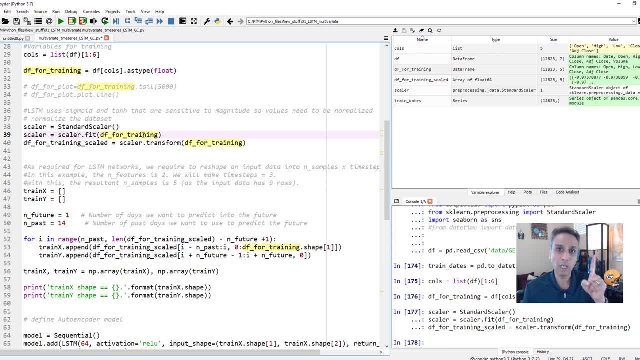 in this example, we could have actually fit This only on one column and then applied it to the transform everything. Okay, just a quick note, but I'll show you another trick to while we are doing inverse transform. Okay, there you go. that deserves one minute, believe me. 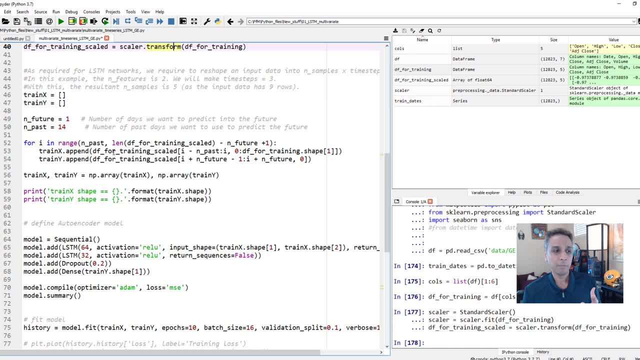 Okay, so now this is the meat of multivariate, because the LSTM part it doesn't care. It just looks at your input shape and then it does the training. But how do you get the input shape ready? It's again. we have done this in almost all of our time series. 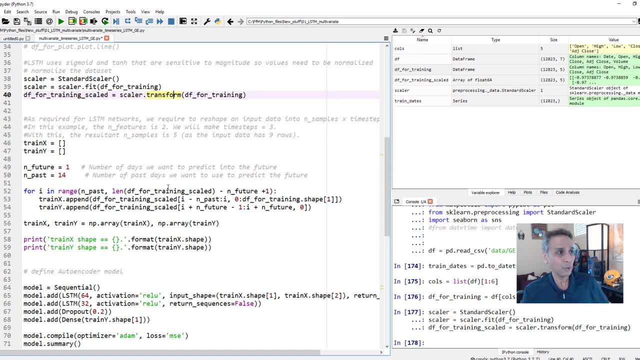 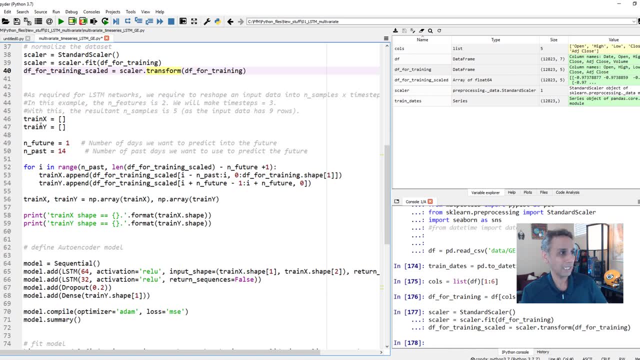 Based. you know videos. So all we're trying to do is, you know, you can write a function for this or you can just do this on the fly. So what we are trying to do is capture our training and the prediction right. So train X is our training series and train Y is the prediction. 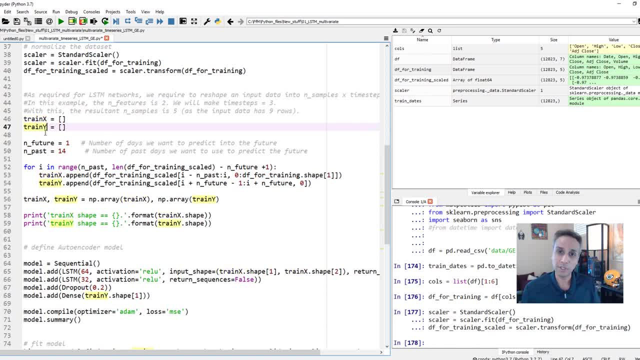 So what is train X and train Y? So this is again time series, which means if I take my first value up to the 10th value As my X, then the 11th value is my Y. it doesn't have to be 11th, you can also say 10th. you know, 21st value is your Y. so you can look forward in future. 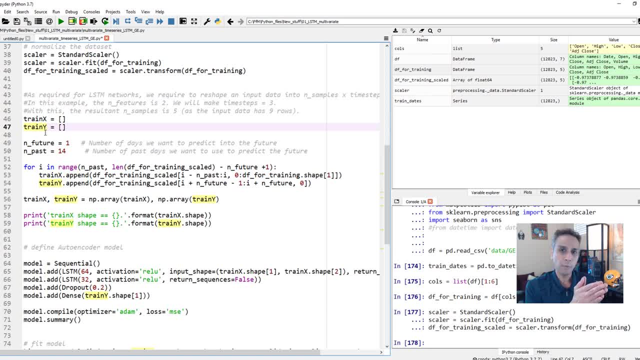 But typically it's customary to look at: okay, I want to use 10 as input and then the next one as output, and then move this by one right: 10 as input, the next one as output. So you can do this as a sliding window and, like I said, it doesn't have to be one you get. your output can be the third, one or fourth one. 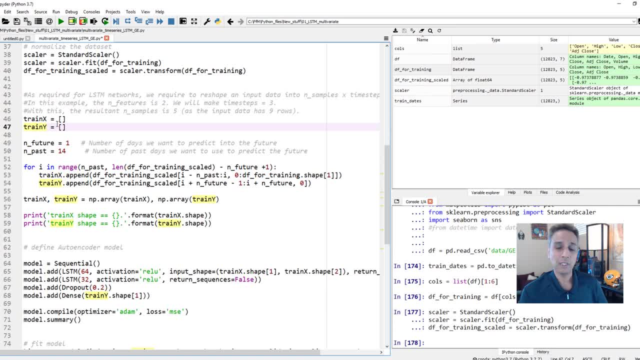 It Uh, Uh And so on. So we are going to capture that, so we are going to reshape our, our five variables that we have, into these chunks and then what the uh, you know value, we are trying to fit it to. Okay, so that's what n future is how, how you know how far in future are you going to predict? 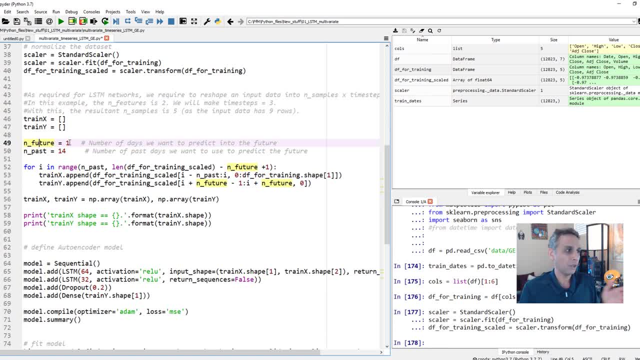 Let me just put one that basically means: okay, go from one to 10. or, in this example, go from one to 14. I want to see two weeks behind, okay, back. And then one to 14, and 15th value is my uh prediction, is the next one. and then go from two to 15, and 16 is the one is my prediction, and so on. so that's exactly what I'm trying to define here and that's what this uh, this, this for loop actually does. so let us uh run these lines. 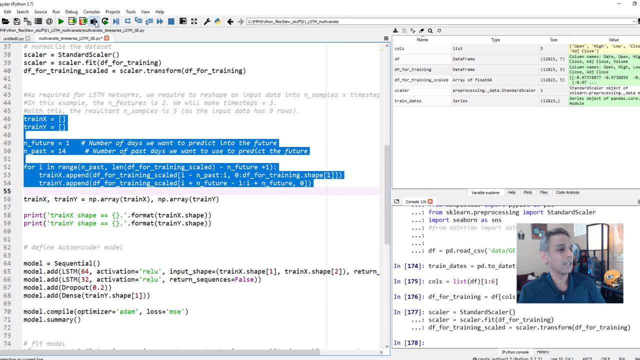 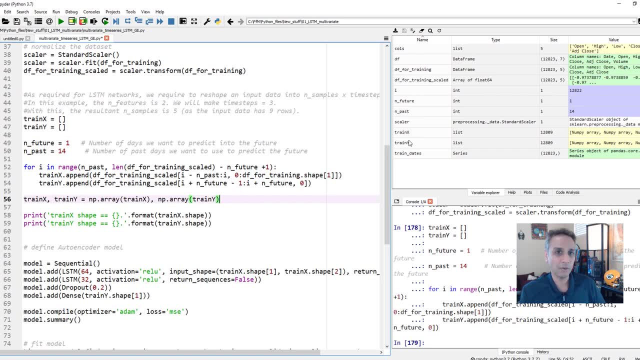 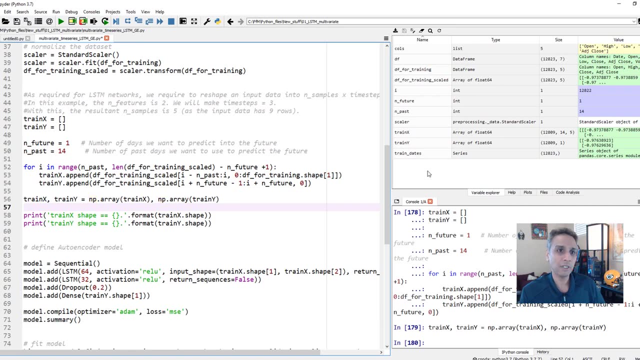 Okay and uh, there you go and now convert this into. if I go back here, you can see my n future. Where is it? Train x and train y? these two are lists, so let's convert them into array. that's all I'm trying to do here and I'll open this in a second. once we convert that into array, it makes it a bit easy for us to see. you see, how my train x is. these many data points. 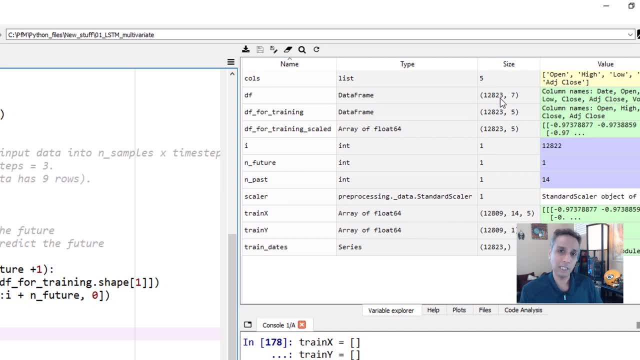 Okay, twelve thousand eight or nine. it's not twelve thousand eight twenty three, because we are holding 14 days or we are uh, so, uh, you have to account for that, okay, so twelve thousand eight or nine, let's go ahead and open it by 14, by five. 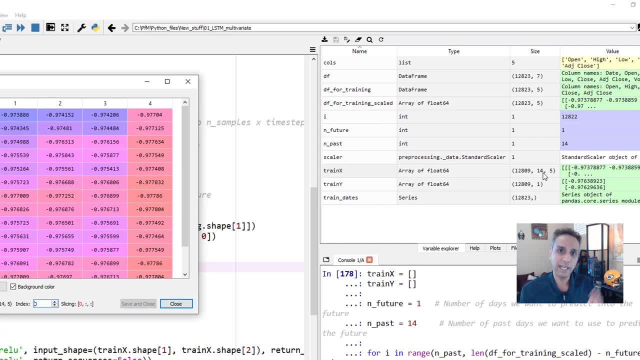 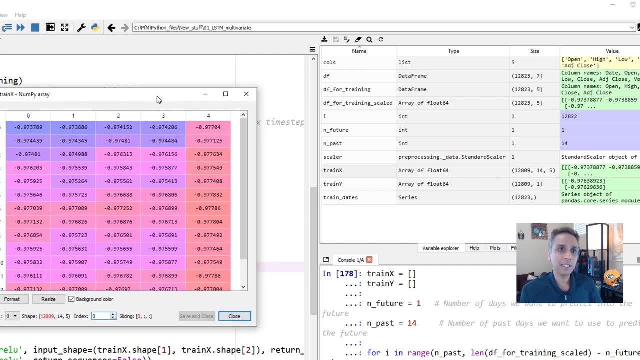 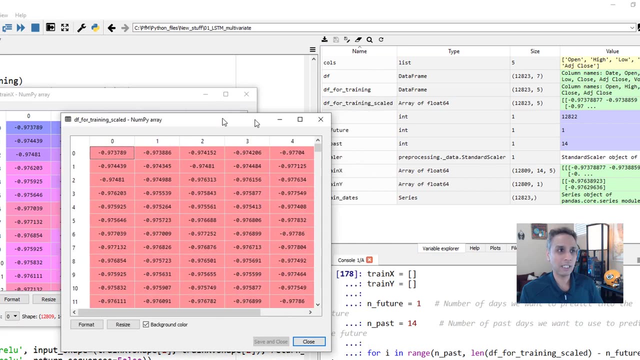 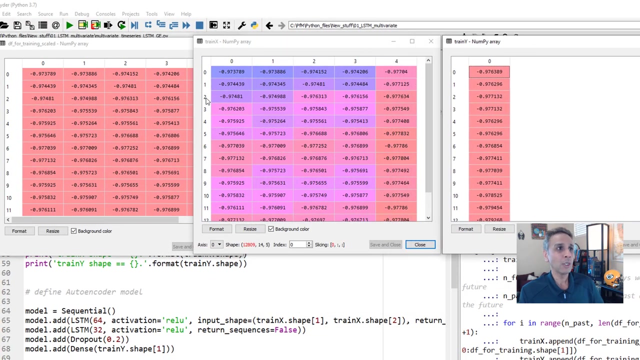 What is this? Four, Fourteen. the fourteen is the fourteen days and, uh, you know that we are looking back and the five is the five variables that we got. okay, now let me open this. this is the key part. everything else should be uh easy. and let's look at df for training scaled. this is the entire data set, this is the training data set, and let's look at the y values right there. okay, so this is variable number one, which is the open. second one is something else, and, and one of these is closed. 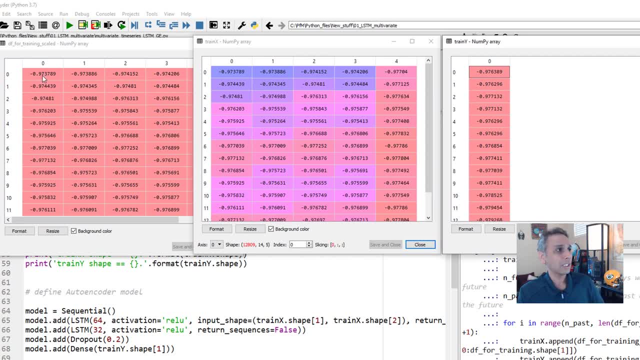 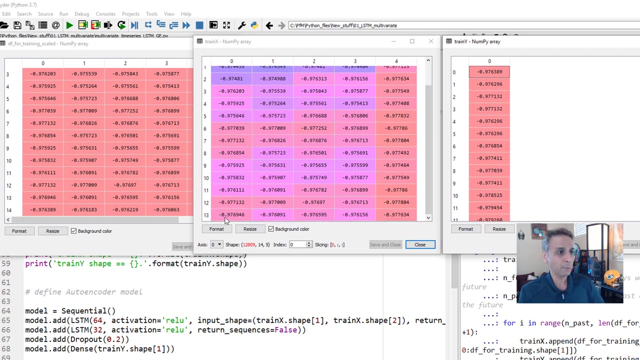 You, you know what those are. so we are starting with negative point nine, seven, three, seven, eight, nine, right, so how far down are we going? thirteen, zero to thirteen, remember, total fourteen points for our x value. so each of this column is going into, uh, into the, into the system, you know, into into our lstm as a training vector. okay, so point nine, seven, nine, seven. so let's go down to thirteenth one. nine, seven, six, nine, four, seven. 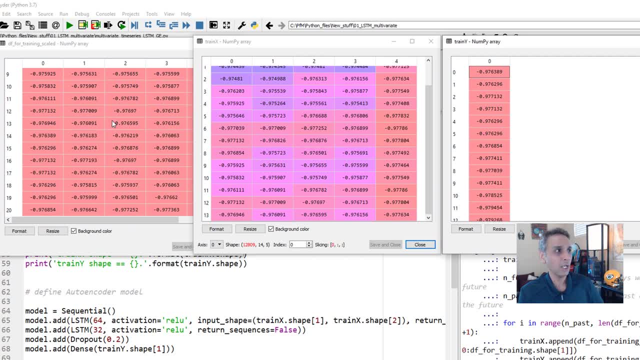 Okay, so point nine, seven, nine, seven. so let's go down to thirteenth one: nine, seven, six, nine, four, seven. So what is the y value for this? what is after? nine, seven, six, nine, four, six. it's nine seven, six, three, eight, nine. that's exactly what the y value is: nine, seven, six, three, eight, nine, right? so for these values, we are predicting the next one and not, if it is just a single variant time series, it would be only this column, because this is multivariate. we have additional four columns. that's the only difference. everything else is exactly the same. 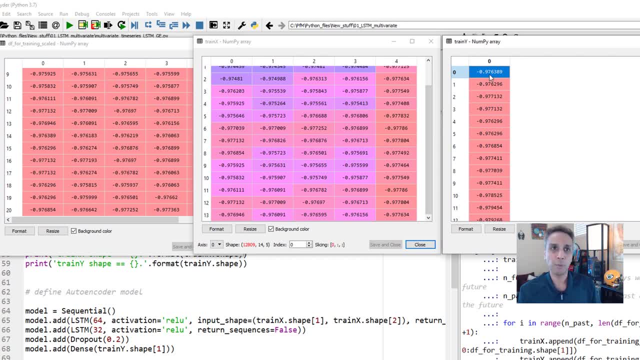 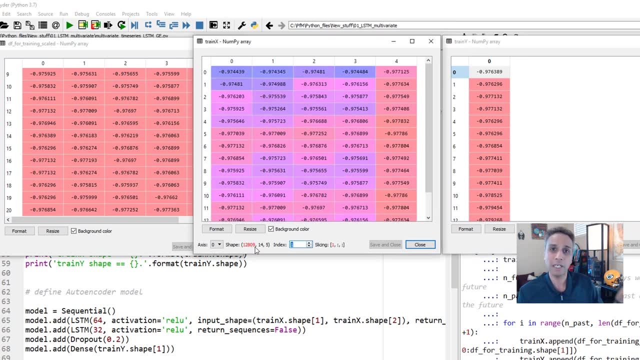 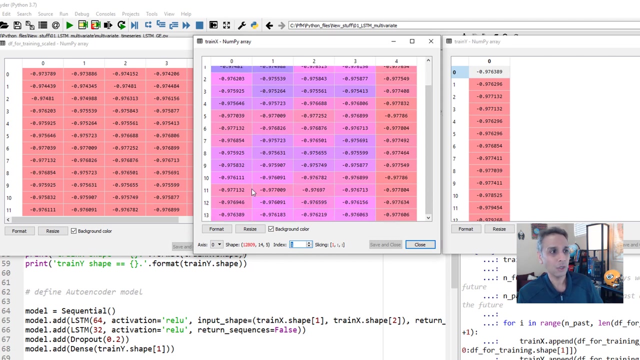 So for this Matrix of values, the prediction is point nine, seven, six, three, eight, nine. for the next matrix, let's go one index up. we have twelve thousand eight, oh, nine such matrices With this prediction, so let me just go by one. that means my starting value now is: let's go back: instead of nine, seven, three, seven, eight, nine, now it is nine, seven, four, four, three, nine, okay, and it goes all the way down to fourteenth value, which is nine, seven, six, three, eight, nine. sorry, 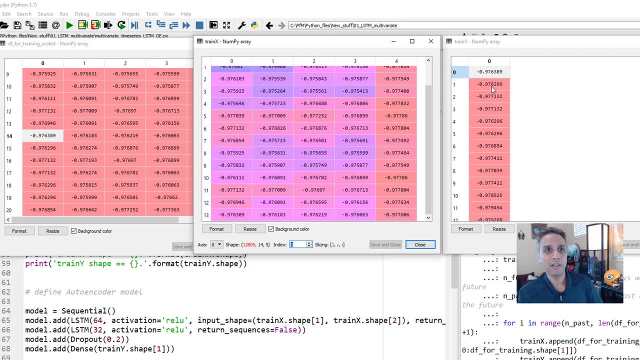 Nine seven, six, three, eight, nine. and what is The prediction Right there? nine seven, six, two, nine six, which is this one? I hope this makes sense. if so, you know everything you needed to. Please don't stop watching the video, because maybe you learn something. but basically, this is it. once you get your multiple variables in this format, you're all set. okay. if it is, if it is a univariate thing, instead of the, instead of this shape being whatever the number of data points. 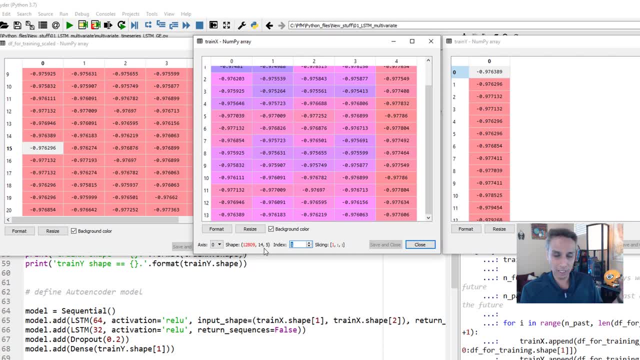 And number of look back, or the days that we are In, Or the sequence size, and this would be one right, because you had one variable. now we have five variables. that's. that's the difference. okay, I think I dwelled on that way too much. I hope it makes sense to you guys. 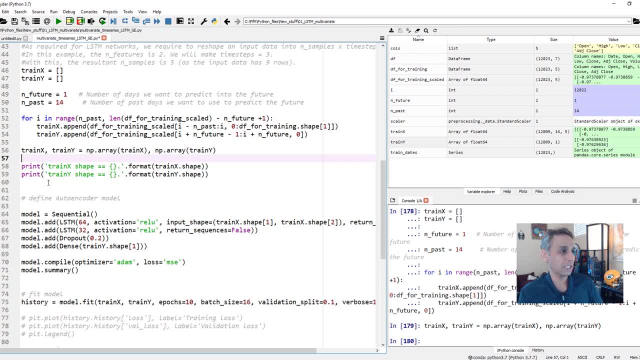 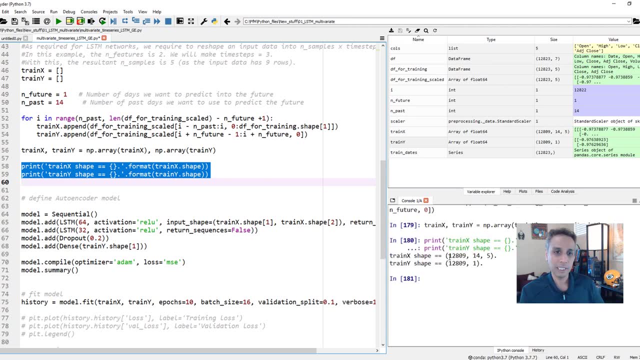 So, once it's done, now you can go ahead and print out what the shape is, in case you cannot read it up there. let's, since it's here, let's go ahead and Do that. and, as you can see, the shape that's going into LSTM, into our neural network, is twelve thousand eight or nine different x values. 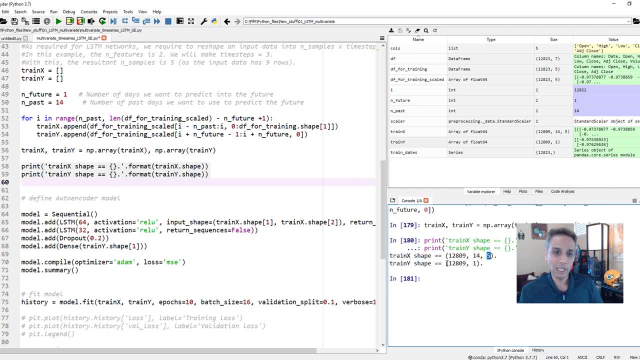 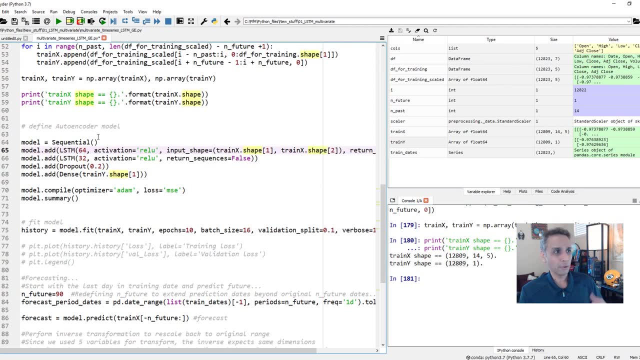 Of size fourteen by five and the y value is twelve thousand eight or nine, we have size one because it's just predicting the day after. okay, How do you put your model together? exactly the way we have done every other model. so in this case we are doing LSTM with sixty four units and my input shape is three, next shape one and three, next shape two. right, so my train x shape one and two is fourteen by five. 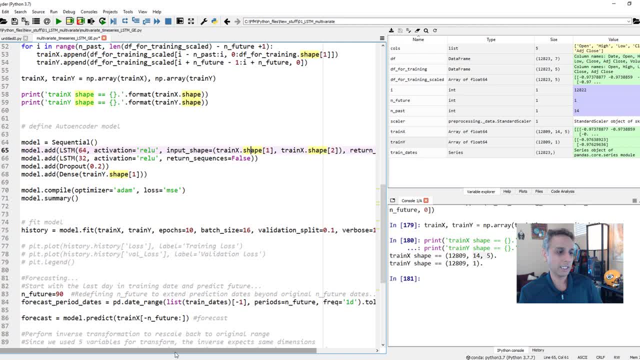 Right there, and This is important, Return sequence is equal to two. True, why? because I want this LSTM to return a sequence for the next LSTM to process. that's why, okay, because I have a stacked LSTM. if you, if you are not including this, then change that to false, okay, otherwise you'll see some errors. 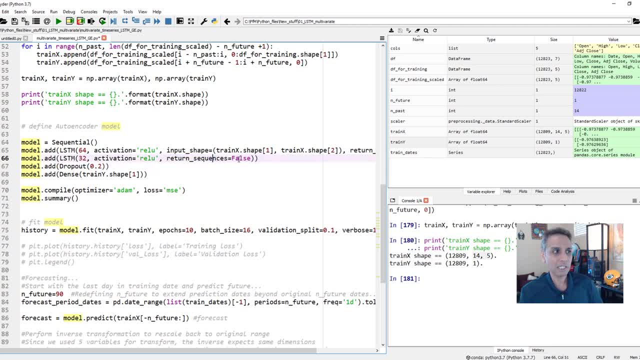 And return sequences for the next one is false because the next layer is just a dropout layer or you can directly go to dense layer, it doesn't matter. but If you say return sequence is equals to false, it's not returning the sequence, it's returning a vector that goes into your dense layer and then 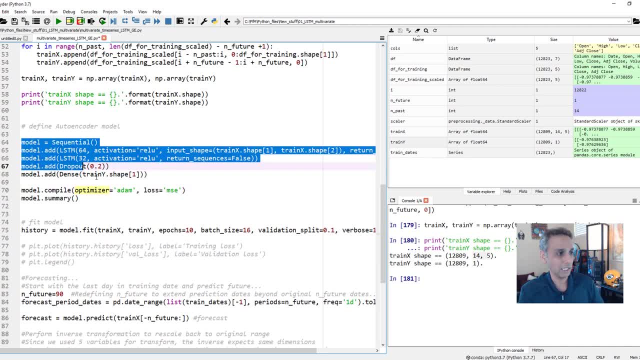 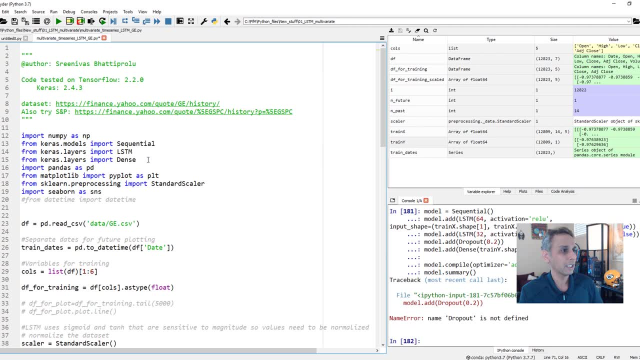 You're compiling it and you're looking at the summary. that's it, okay, so let's go ahead and print the summary. A dropout is not defined. did I remove it, Layers? let's go ahead and include it. I don't know why I did that. 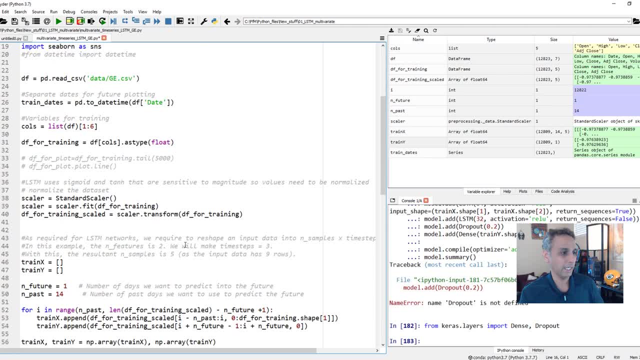 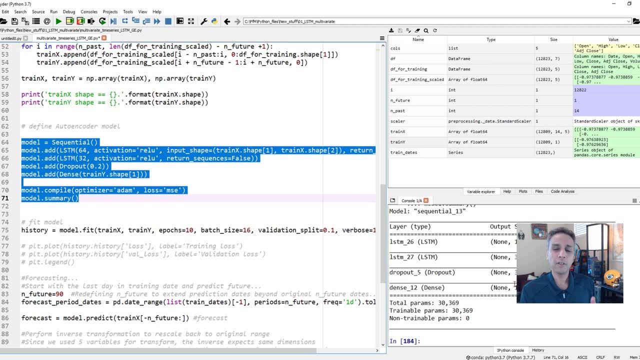 Sorry about that. so let's include dropout, okay. so now let's come back And run this one more time. there you go. so okay, here is our structure: thirty thousand parameters. that's fine, it should be fine, Okay, Okay, Okay, It should be pretty quick, okay. 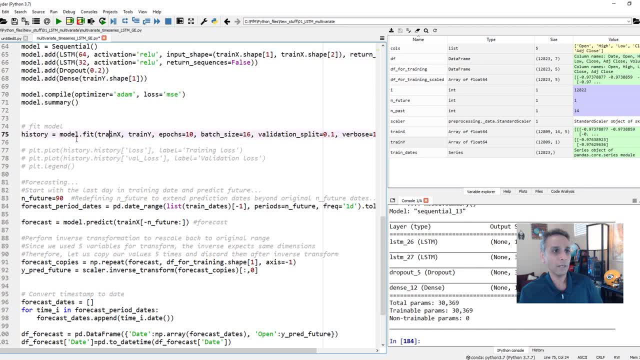 Even on my system, but I'll pause this in a second. so now I'm doing no tricks again, just model that fit training strain. why? exactly the same that we normally do. let's only do ten Epox for now. okay, let's run this And I'll pause this and I'll continue in a second. 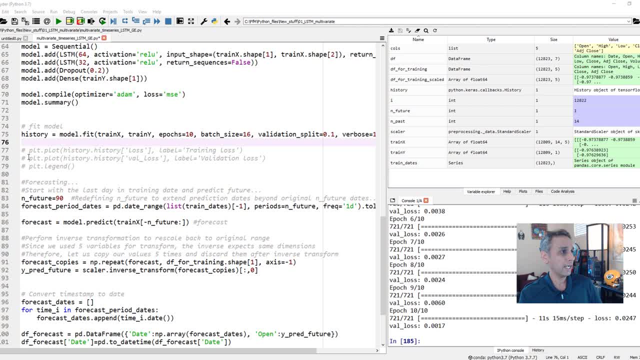 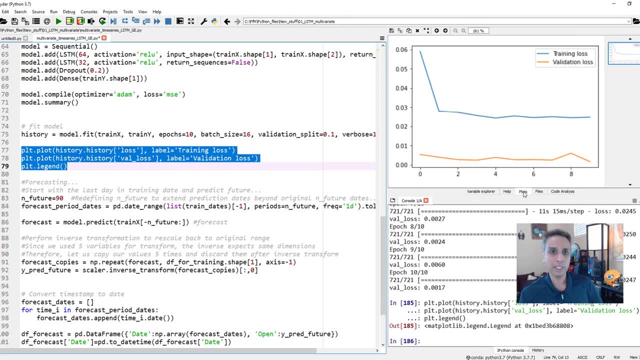 Okay, so there you go. it's done after a few seconds, so let's go ahead. and I commented just for some reason. but let's go ahead and uncommitted, and have a quick look at how the training went. training went Okay. I guess that's okay. Let's now go ahead and forecast it. Now, how do we do? 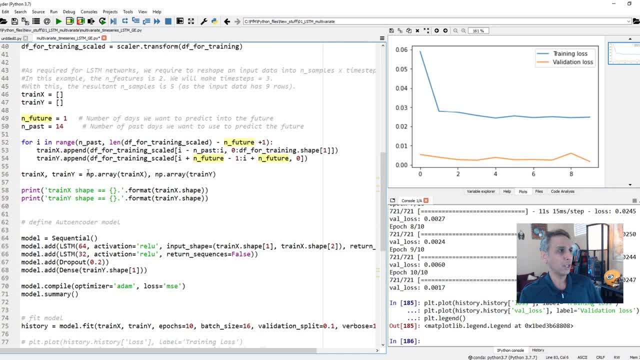 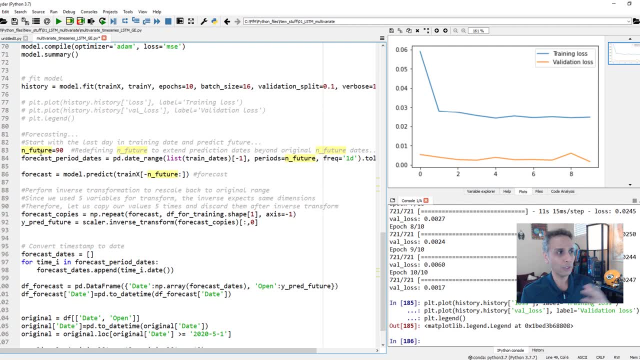 that I defined this in future again. I know I used it here and I defined it like as one. I could have used a different variable. When you're writing your code, change it to a different variable, because I just don't want to forecast one more. I want to forecast like 90 days, like three months. 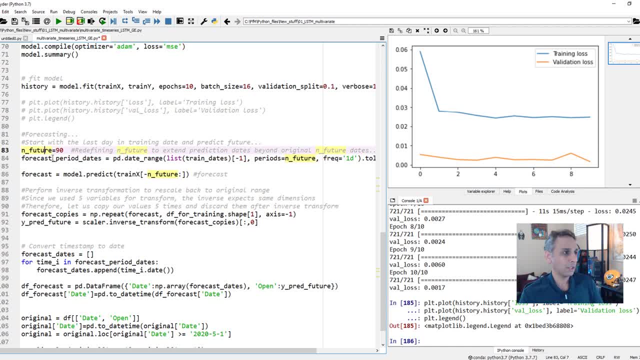 and then just plot it so we can have a quick look at it. Okay, So that's what I'm trying to do here. So just my future days. number of days is 90. And then all I'm trying to do is extract the dates. 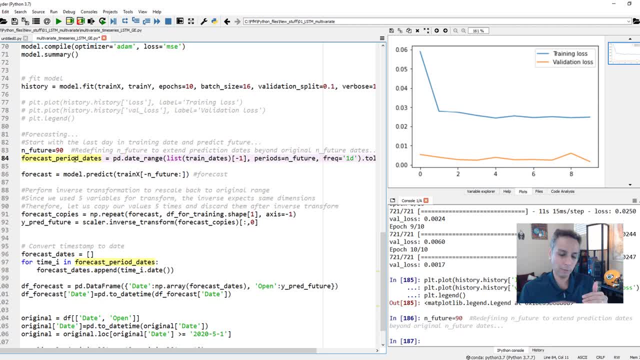 Okay, What would be my future dates? Because when I want to plot, I want to plot the forecasting along with the original right. So I need to extract the right dates. So the way I'm doing that is okay. take the current date minus one, Okay. So that day and then. 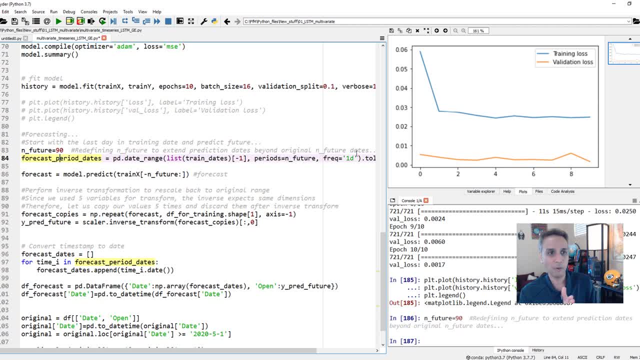 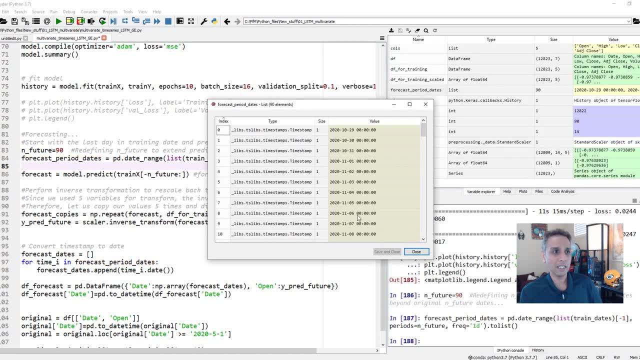 go to 90 days in future, with a frequency of one day. Okay, So that's exactly what this does, And if you look at the forecast period dates, it's just a list of all the dates, starting with October 29th, which apparently was the last day where the training stopped, And then we are going. 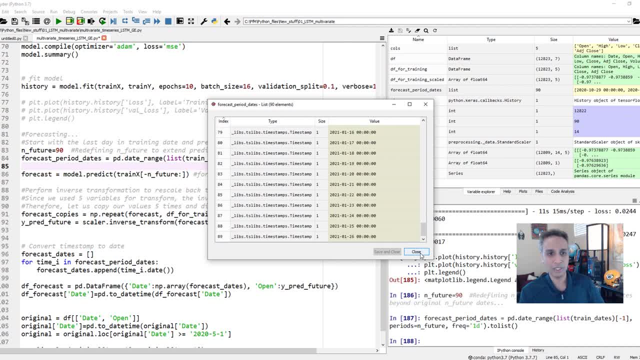 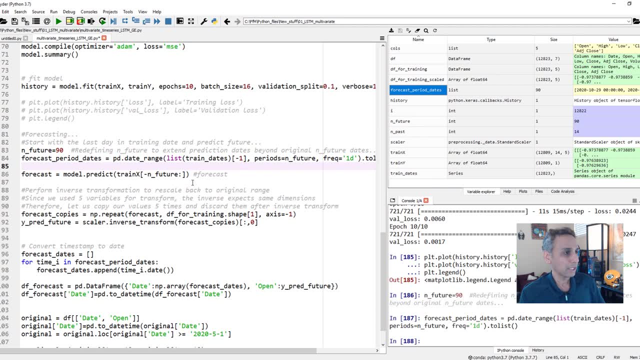 all the way to, I don't know- December or 2021, January 26th, if we all don't die by then of coronavirus. So sorry for the grim note over there, But anyway, let's Get back to a more positive tone. So forecast, what's my forecast? It's just modelpredict. 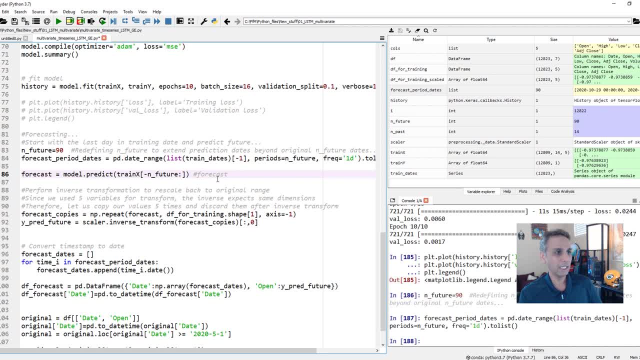 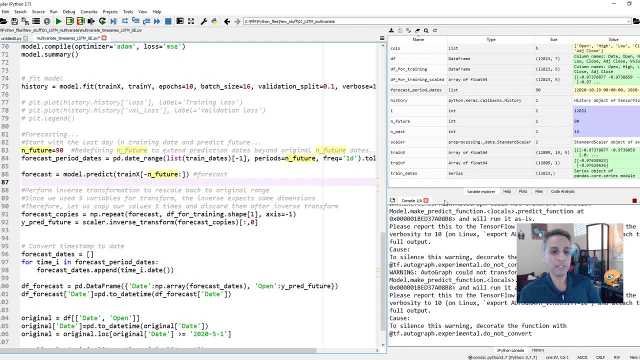 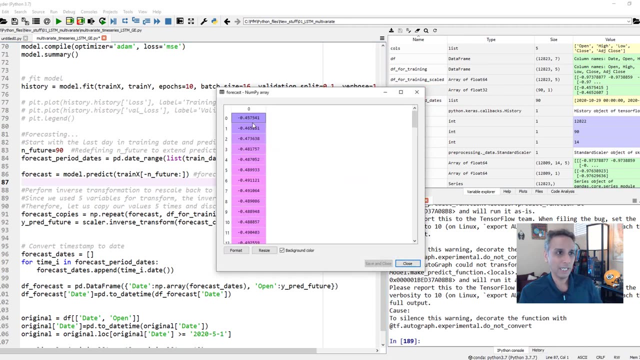 Okay, Train X, from what is my end future number of It's just one, Okay, So let's go ahead and forecast right there, And you'll see that our forecast is of the size 90 by one. Okay, So we are just having a single column right there. So that's my forecast. Okay, Now here comes the trick. 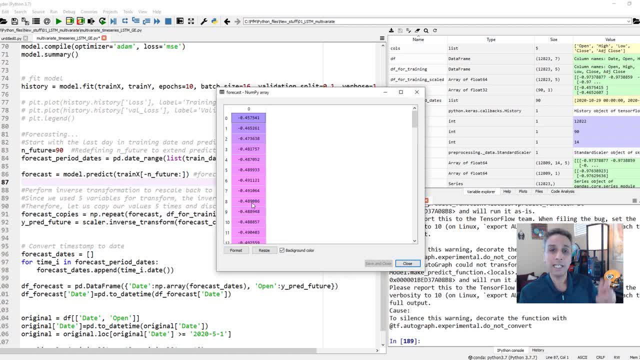 So if I look at the forecast, it's all again in the scaled space, right? Remember, we scaled it using a standard scaler. Now I want the original numbers back. What is the actual stock price? This is not the stock price. This is the normalized or scaled values. I should say So for that. 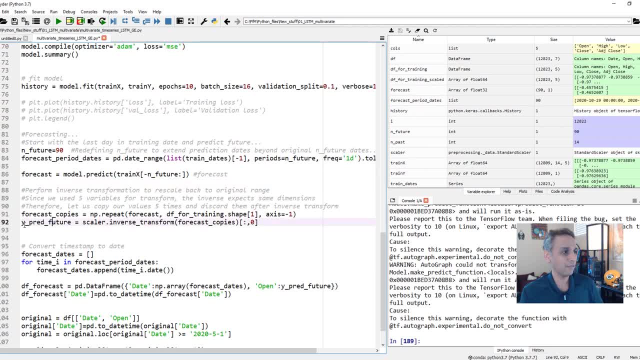 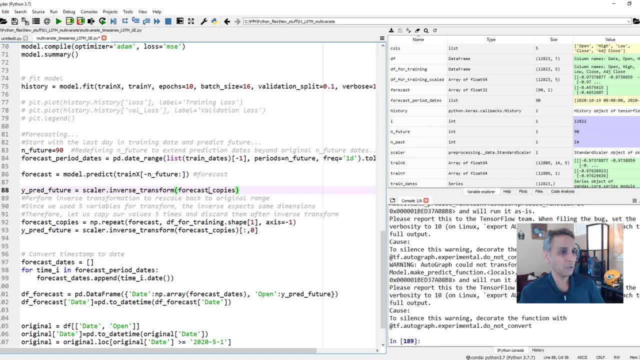 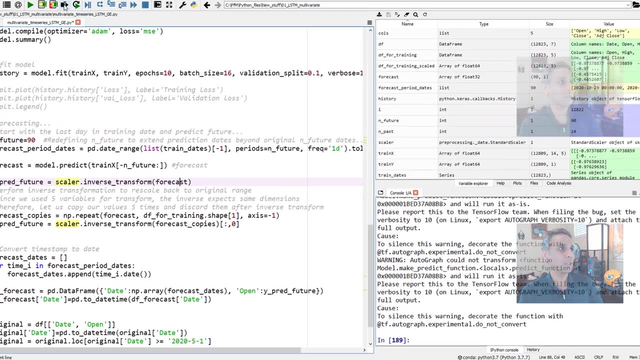 if I just do inverse transform, for example, I think this makes sense. Let's go ahead and do that. If I just do inverse transform- right, I mean, this is how you do it- Scalerinverse transform forecast- It's going to throw an error saying okay, non-broadcast output. 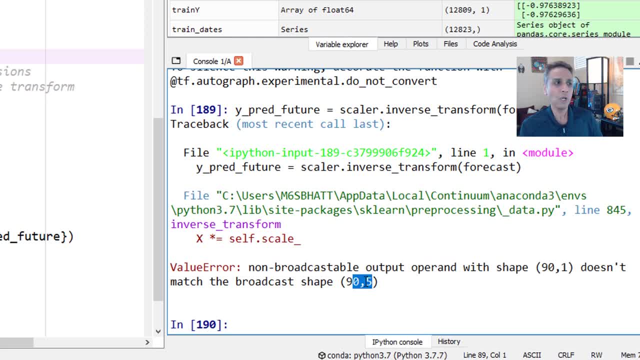 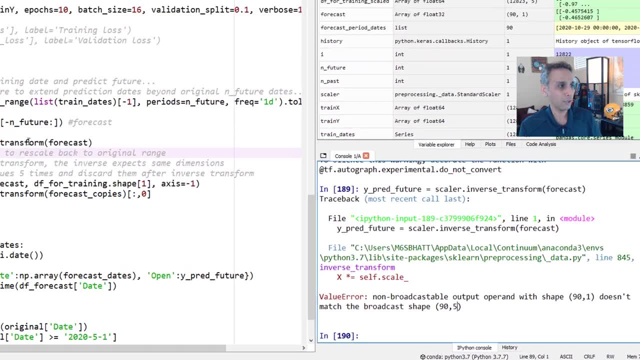 offering 91 doesn't match the broadcast shape 95. What that means is, hey, you only have a single column, but when you scaled it you had five columns right. So this is what I was talking about. So for that, I mean there are a few ways you can do. I mean you could have actually gone. 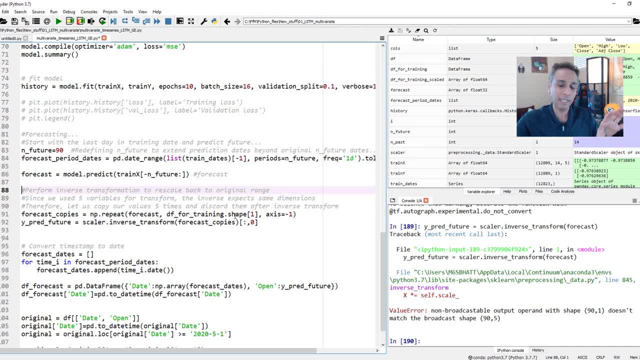 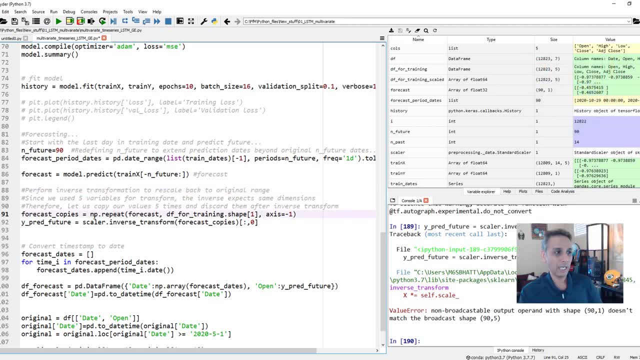 back to original data frame and copied those or the scaled data frame, copied those values for the other variables. many tricks. What I chose to do here is: I just used nprepeat to repeat that column. how many times For training shape one which is nothing but five, right. So df for training. 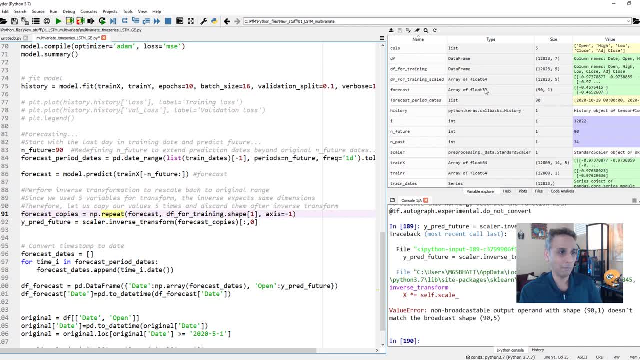 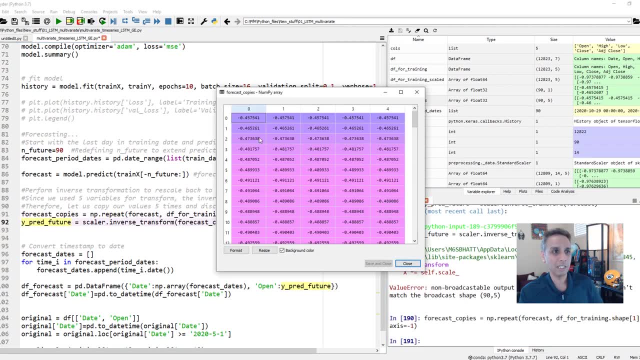 df for training. shape one is five. okay, Five variables, Or you can just type five right here, It doesn't matter. So let's just do forecast copies, forecast copies. If I open this, it's just the same thing It copied five times, And then I'm going to drop everything after. 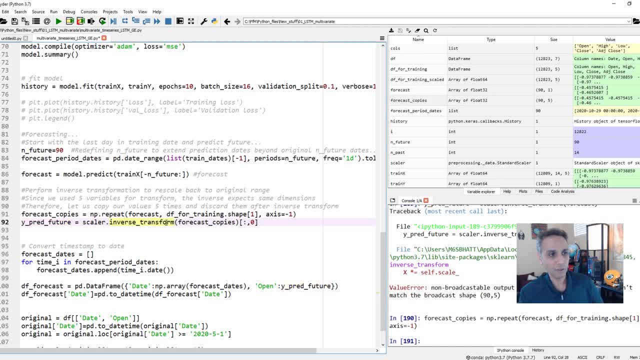 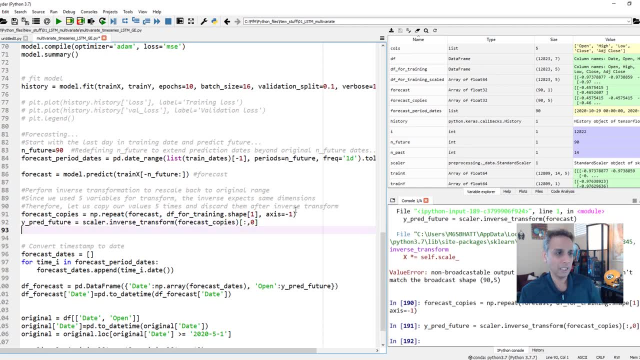 inverse transform. You see, that's exactly what I'm doing. I'm doing inverse transform, but I'm only looking at the zeroth one, which means I don't care about everything else. It's a weird way of doing things, but it works Okay. so now I have my y predict future. So this: 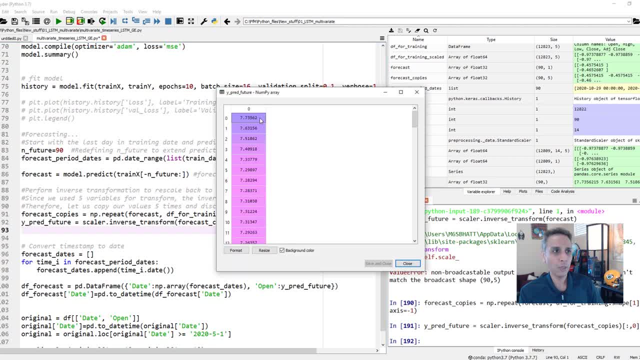 is the predictions. These are the predicted values. There you go. I still have one column, and now you see how the values are in real dollars and not like negative zero point something. So this is it. This is our prediction. Now all we have to do is attach this to the right dates. 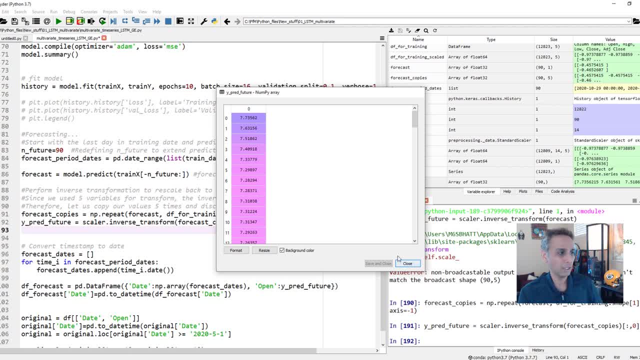 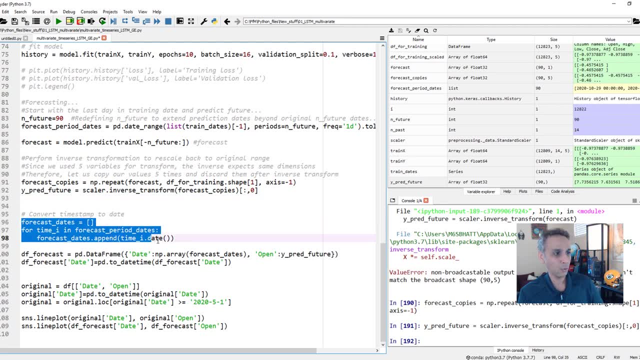 and plot this With the original data. That's all we're trying to do now. Okay, so my forecast dates for time in the forecast period dates: Okay, go ahead and append this, So we'll have that part And then we. 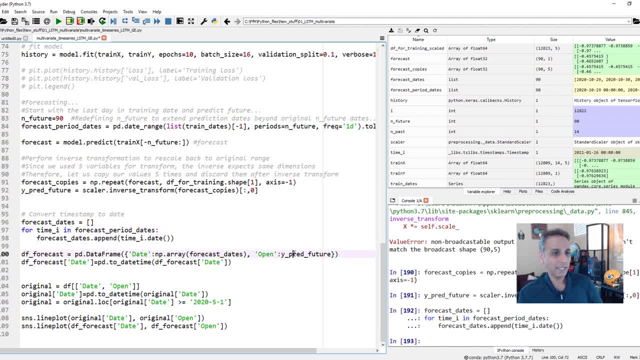 are going to capture that- the forecast dates okay, And y predict future- both of this into a single data frame. And you see how I define this in a dictionary where my column name is date and here the column name is open. 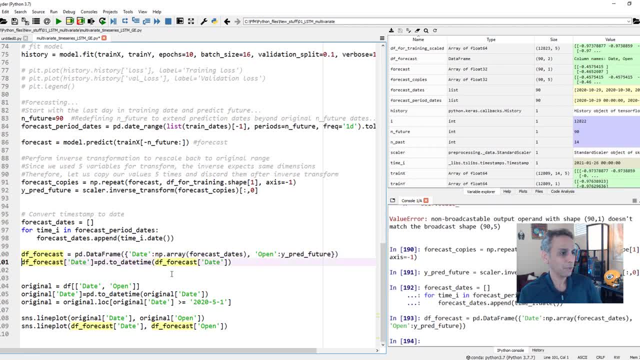 So, again, I hope you're pretty good at pandas. So there you go. So my data frame with forecast is this: and now I'm converting my date back into the date time format. You may think like, okay, why are you doing this? And you could have handled things in a better way. 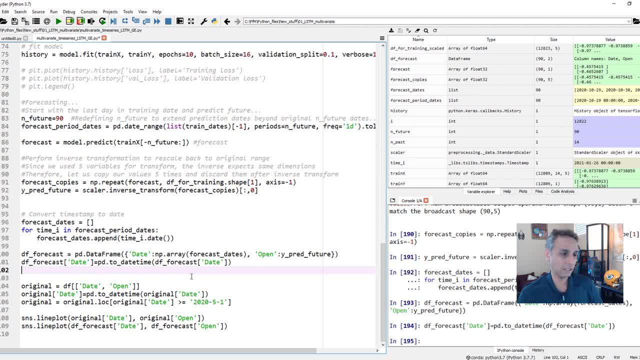 Of course, we could have handled things in a better way. This is something I put together pretty quickly and I was writing stuff as I was going along, So if you are a better planner, you probably have a good idea of this, and we could have reduced this code by a few more lines. Okay, so now we have our data frame for forecast, right? 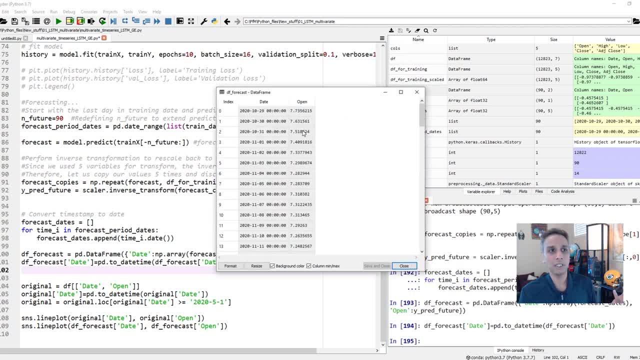 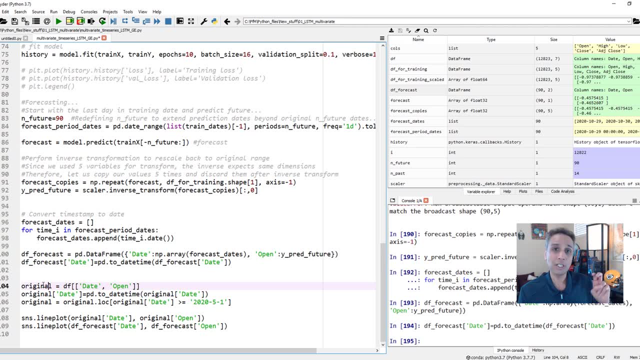 here and you have the date and you have the opening, predicted values. We could have just said: opening, predicted. And now let's do exactly the same with our original data frame, right? So what is our original data? Our original data is in DF, right there? 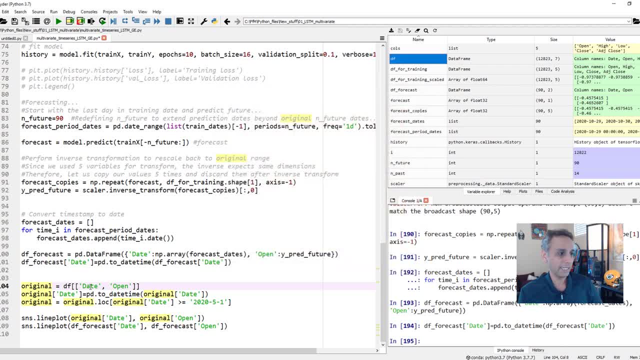 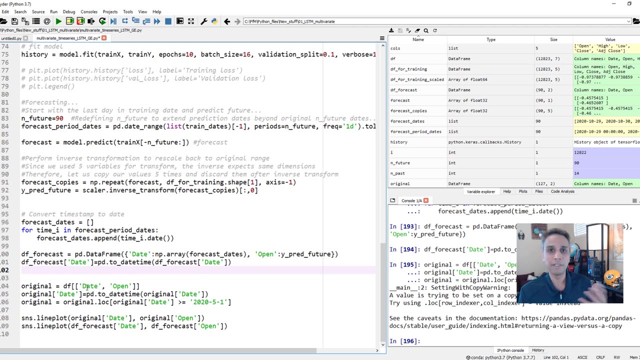 This is our original data and we just need to extract the date and opening time and let's go ahead and do all of these. okay, so there you go. all I'm trying to do is basically get original data from the original data frame. okay, and only the two columns: date. 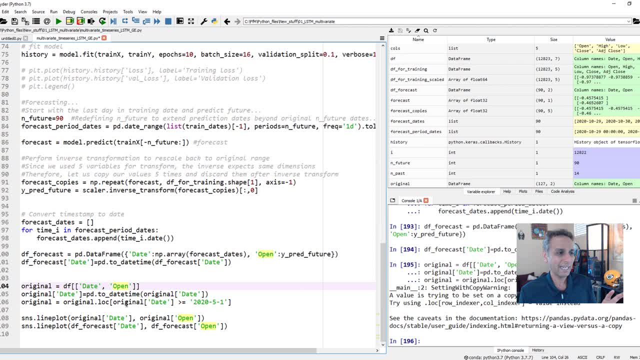 and open. this is what we need. that's it. we don't need anything else. and here I'm just looking at everything that's after May 1st 2020. otherwise the forecast is that tiny, and then the entire graph and it's tough to see things. so this is only 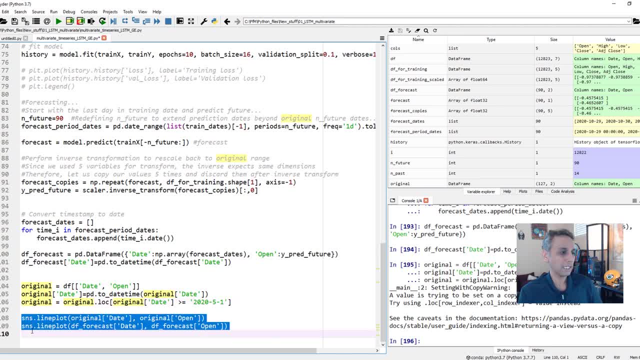 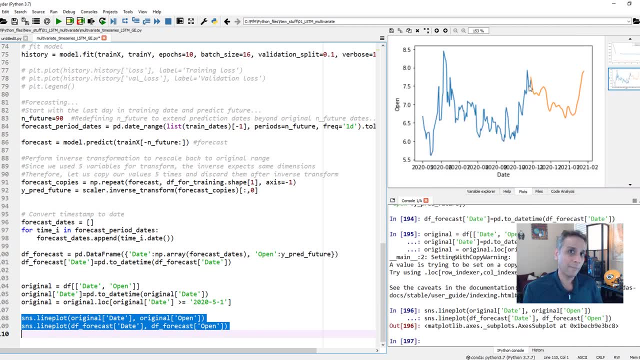 for visualization purposes. okay, now let's go ahead and plot it again. I'm using seaborne, you can use piplot for plotting. so here it is. let's see how good it is. that's not bad, I mean, I could have actually overlapped some of these. 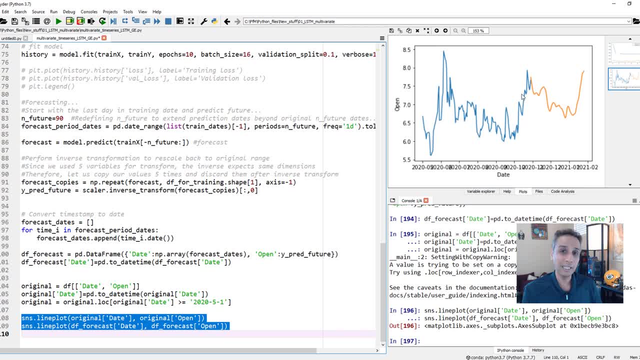 and you can see how the prediction actually goes. I leave that exercise to you. in fact, you can predict all the way from the beginning to here and then see how it continues, but anyway. so here is the original data and here is the forecast for I don't know 60 days- how many. 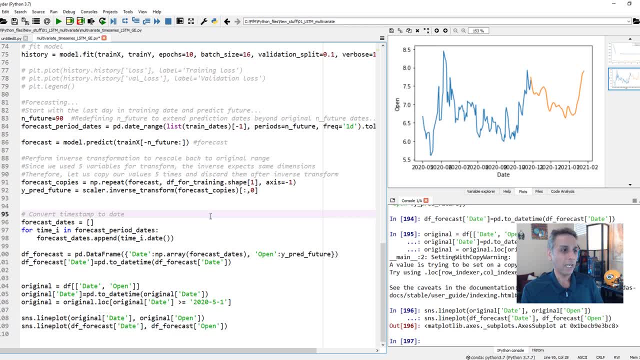 you're up future 90 days in future, okay. so I hope now you know how to work with multivariate data set. just like linear regression, multilinear regression, nothing, it's pretty much the same thing. you just get the data in the right format. same thing here: linear, you know, or sorry, you univariate or multivariate. 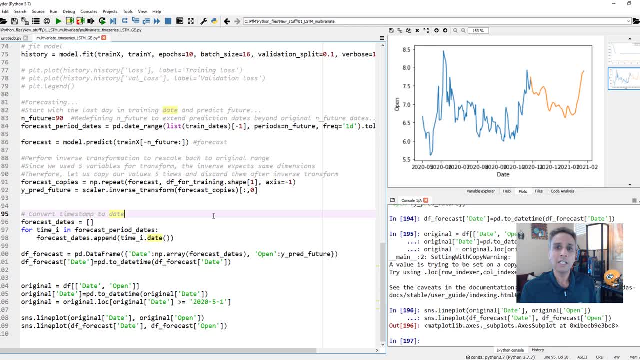 you just get the data in the right format, then you're all set okay. so thank you very much for watching this video and again, keep requesting other stuff and if I have time and if I have skills in that field, I'll definitely make a video on that topic or I'll do my research online and I'll digest the 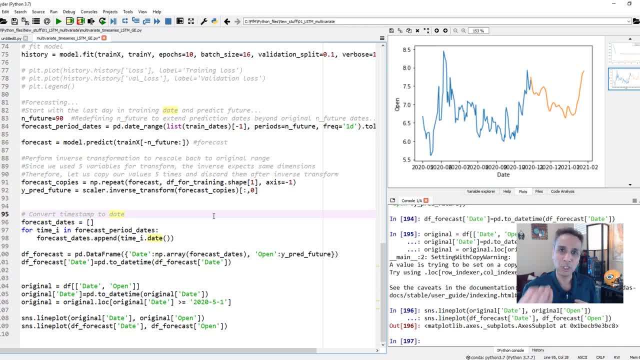 information and regurgitate to you in digestible chunks so you can understand it, but please do leave feedback in terms of if you want something you know that you're struggling with and if you think I can help you out. thanks again, please do subscribe.